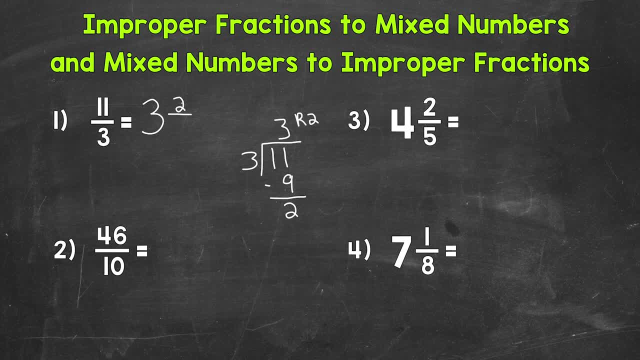 So that remainder is going to be our numerator, And then we use the original denominator of 3 for the denominator of our fractional part of the mixed number. Always check to see if you can simplify the fractional part of a mixed number. Two thirds is in simplest form. 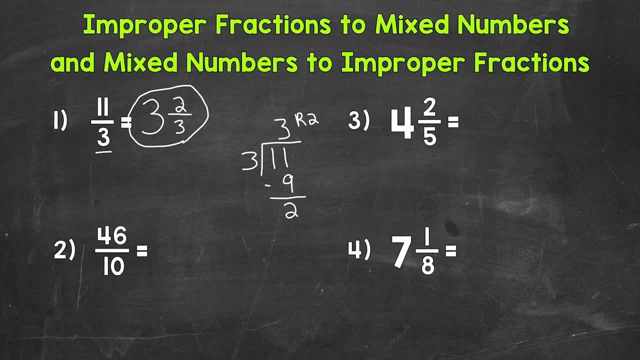 So we are done. Let's move on to number 2, where we have 46 tenths. So again, we need to divide 46, the numerator divided by 10, the denominator. Let's do that, Let's write this one out as well. 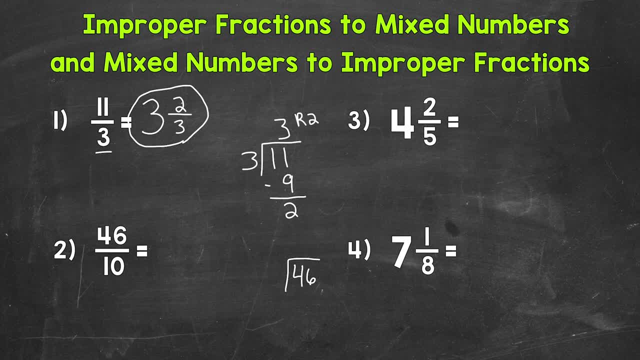 So we have 46 divided by 10.. So we need to think how many whole groups of 10 do we have in 46?? Well, 4. That gets us to 40. Four whole groups of 10. So that's our whole number for our mixed number. 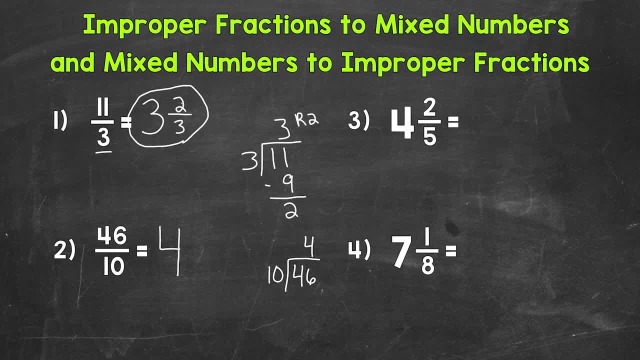 Now we do not hit 46 exactly. We have a remainder, something left over. So 4 times 10 is 40.. 4 times 10 is 40. Let's subtract, Let's subtract And we get 6.. 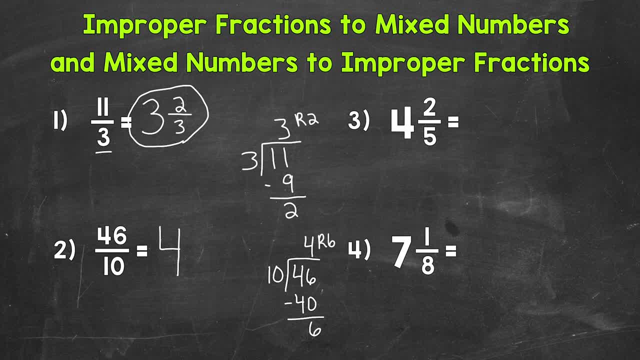 So a remainder of 6.. That remainder is our numerator, And we use our original denominator of 10 for our mixed number as well. Now the fractional part of the mixed number for number 2 can be simplified. We have a greatest common factor of 2 for the 6 and 10 here. 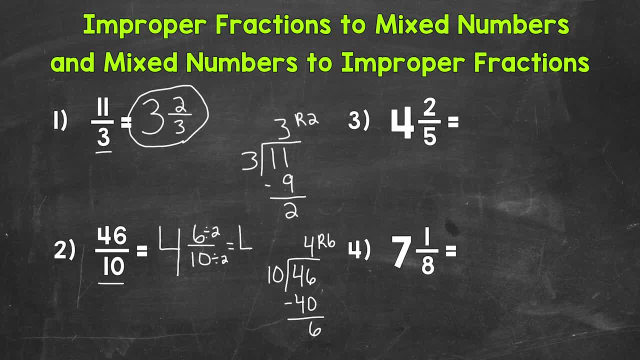 So we can divide both of these by 2.. and we get 4.. 6 divided by 2 is 3.. 10 divided by 2 is 5.. So our final simplified mixed number is 4 and 3, fifths. Let's move on to numbers 3 and 4, where we have mixed numbers and we are going. 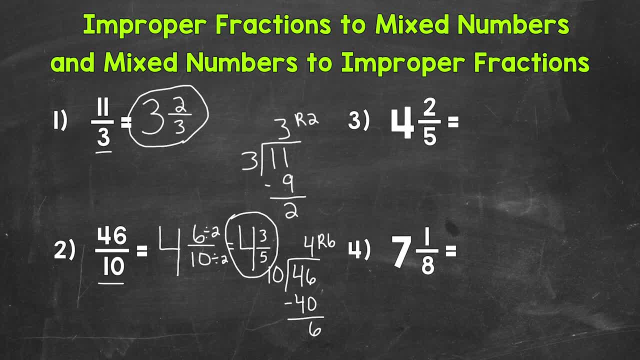 to convert them to improper fractions. And we do this by multiplying and then adding. So I'll show you the process first and then show you how and why it works. So we start at the bottom and work our way up, We multiply and then add. So 5 times 4 is 20, plus 2 is 22.. So that is our numerator. 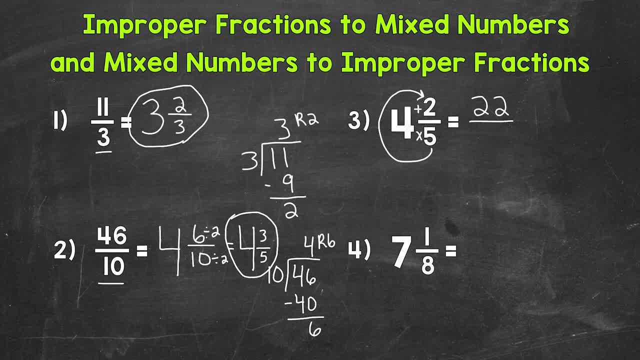 Again we did 5 times 4 is 20, plus 2 is 22.. We can keep the denominator of 5 the same, So 22 fifths is our improper fraction. And the reason this works is because let's think of 4 wholes. Now I'm going to write out 4 wholes as a fraction. 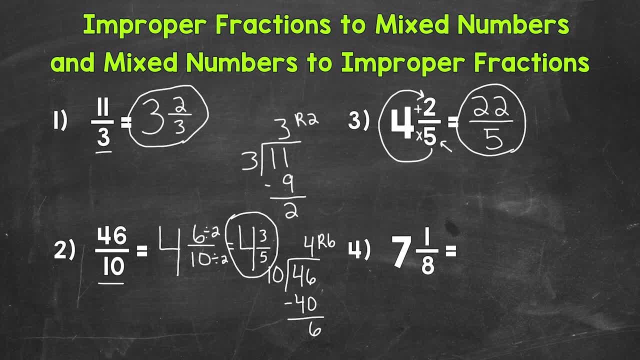 using this denominator of 5.. So, for example, 1 whole would be 5 over 5.. And I'm picking 5 because that's our denominator, So this is going to make it easier Just using that denominator. Now we have 4 wholes, So 5 fifths, 5 over 5, plus 5 over 5.. That would 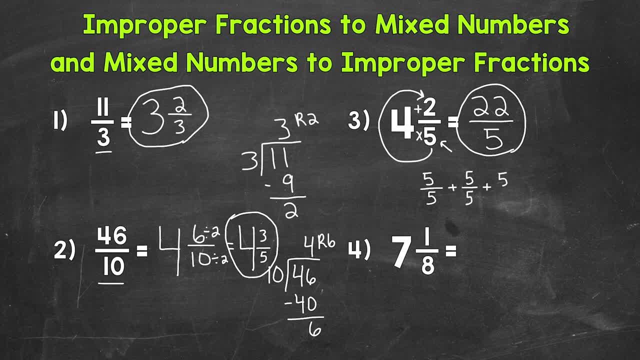 represent 2 wholes, but we need 4.. So let's do another one. There's 3 wholes, 4 wholes plus our fractional part of 2 fifths. So these right here represent the 4 wholes. Then we have the fractional part 2 fifths. So let's add all of these up. 5 plus 5 is 10, plus 5 is 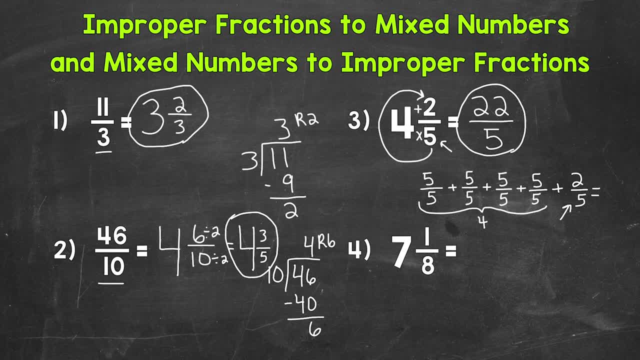 15, plus 5 is 20, plus 2 is 22.. And our denominator is 5.. So we can see that we got 22 fifths. Now, using this method right here is a lot quicker. It's a shorter way than writing everything out. 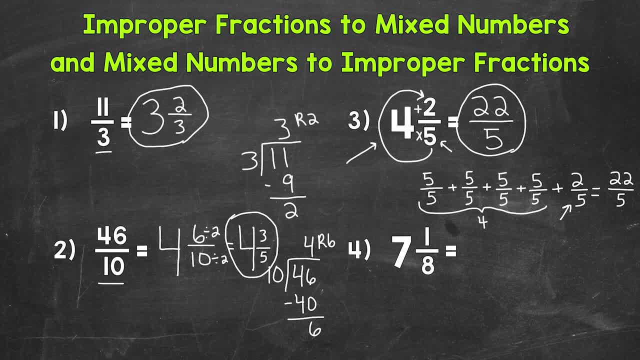 So again, multiply and then add. Let's try another one and move on to number 4, where we have 7 and 1 eighth. So we start at the bottom and work our way up, We multiply and then add. So 8 times 7 is 56,. 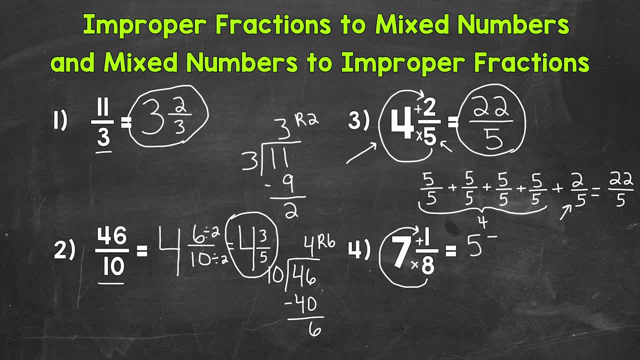 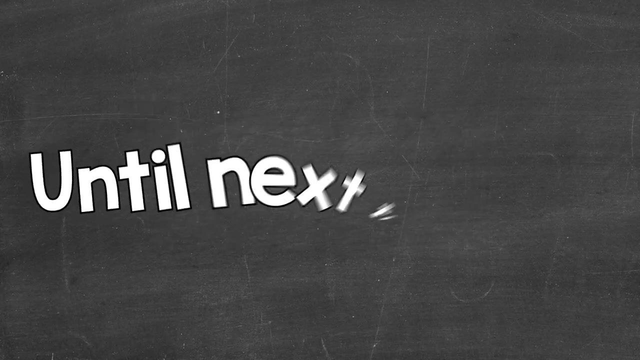 plus 1 is 57.. And then we keep our denominator of 8.. So 57 eighths for number 4.. There you have it. There's how you convert improper fractions to mixed numbers and mixed numbers to improper fractions. I hope that helped. Thanks so much for watching. Until next time, peace.